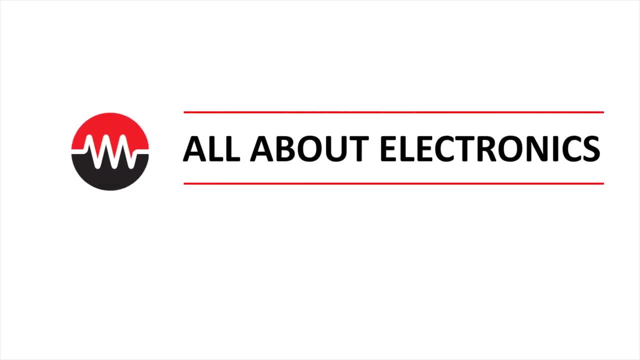 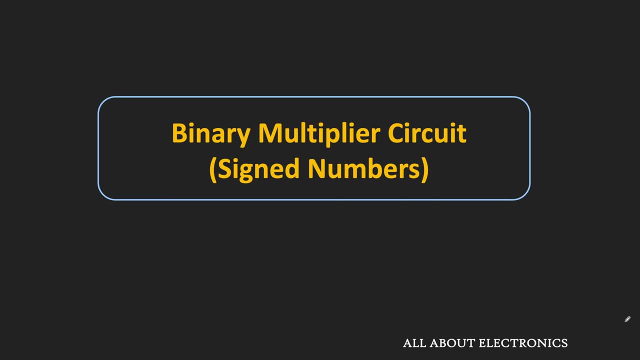 Hey friends, welcome to the YouTube channel ALL ABOUT ELECTRONICS. So in the previous video we have seen the circuit for the array multiplier or the combinational multiplier. So using that circuit we can multiply the unsigned binary numbers. But in the real world we are also dealing with the negative numbers. 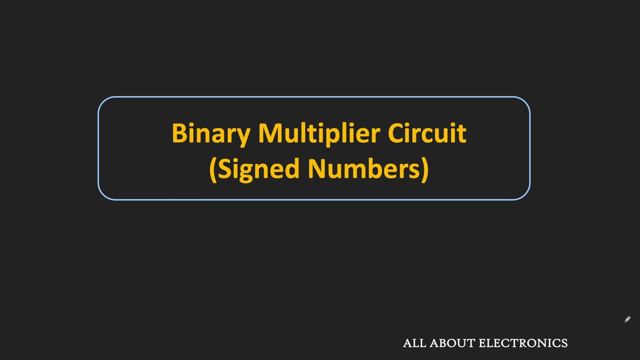 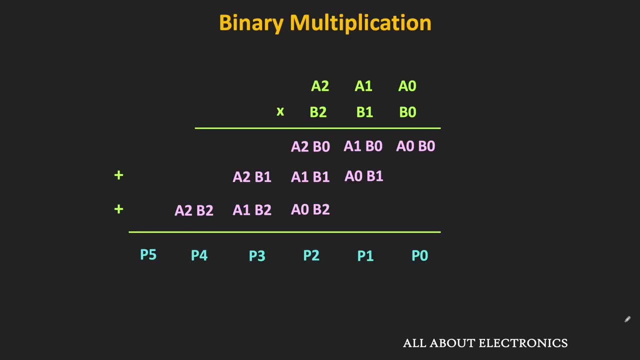 So in this video let's see how to design a multiplier circuit which can multiply the signed binary numbers. So in the earlier video we have already seen the multiplication procedure for the signed binary numbers. So in case of the signed binary numbers we need to extend the signed bit of each partial. 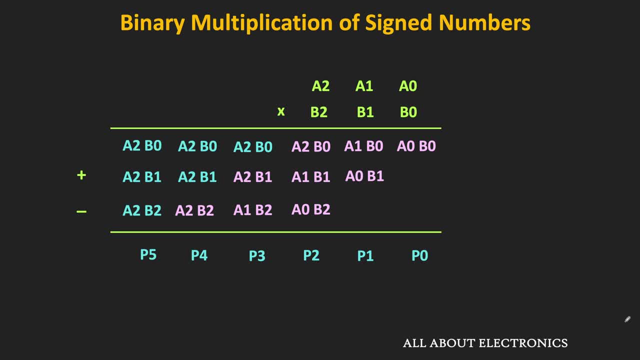 product upto the 2n bits, And we have also seen that in case of the signed binary multiplication we need to subtract the last partial product. That means the multiplication of the signed binary numbers. The signed binary numbers consist of two additional steps. 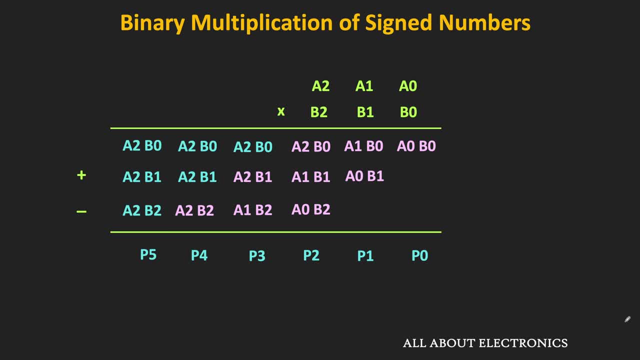 That is, the extension of the signed bit of each partial product upto the 2n bits And the subtraction of the last partial product. So the subtraction of this last partial product is equivalent of taking the 2's compliment of this last partial product. 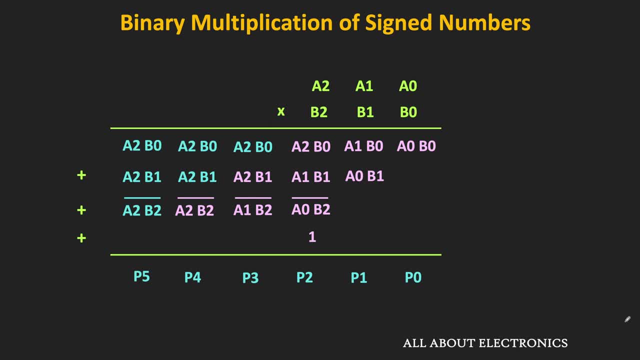 So here the same thing is shown for the 3 bit numbers. So, as you know, taking the 2's complement of number is equivalent of taking the 1's complement of the number followed by the addition of the 2.. Yes, So for the last partial product the same thing is shown over here. 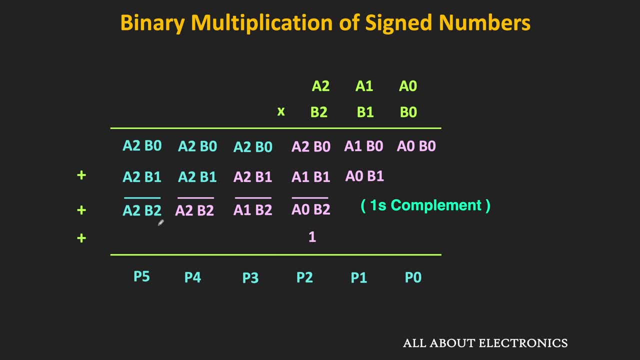 So, as you know, for the ones complement we need to replace zeros by one and ones by zero in the number. So basically we need to complement each bit And then this one is added to get the equivalent two's complement number. 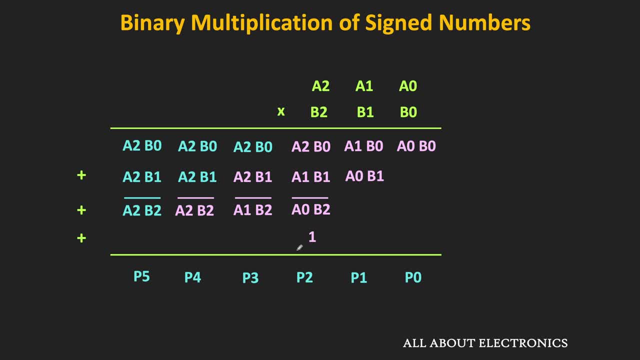 So in the earlier video of the sine binary multiplication I have mentioned that we need to take the two's complement of the last partial product only when the multiplier is the negative number. For example, we need to take this last step whenever this multiplier- B2, B1, B0- is negative. 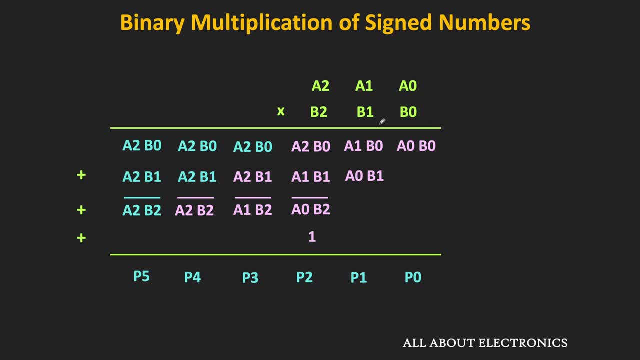 number. But this method will also work even if the multiplier is positive. So if the multiplier is positive, then this bit B2, or the MSB of this number will be zero. So in that case, all these bits, ie A2, B2'. 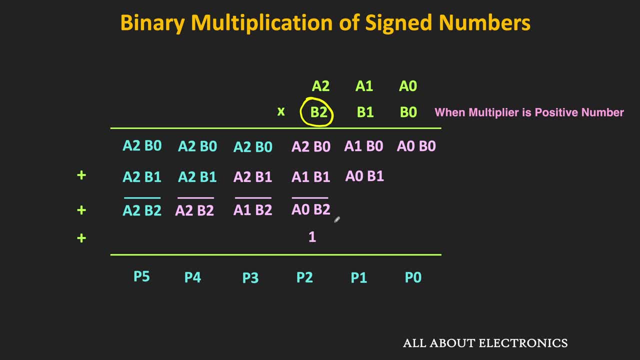 A1- B2' and A0- B2' will be 1.. That means at all those positions we will have 1111.. And when we add 1 to it, then all the bits at the corresponding positions will become zero. 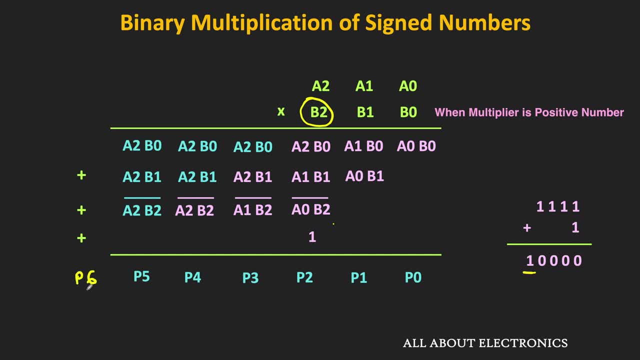 And this one will get shifted to the P6 position. So here we can ignore that bit, Because here we are only concerned about the first 6 bits, That is, from P0 to P5.. That means in this method, Whenever the multiplier is positive, then this B2 bit will be zero. 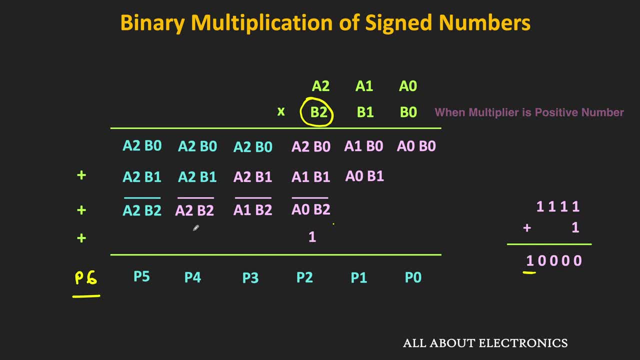 And because of that this last partial product will get vanished And therefore this method will work, even if the multiplier is positive or the negative. So now let's see how to implement the same thing in the digital circuit. So if you want to implement the same thing in the digital circuit, then compared to the 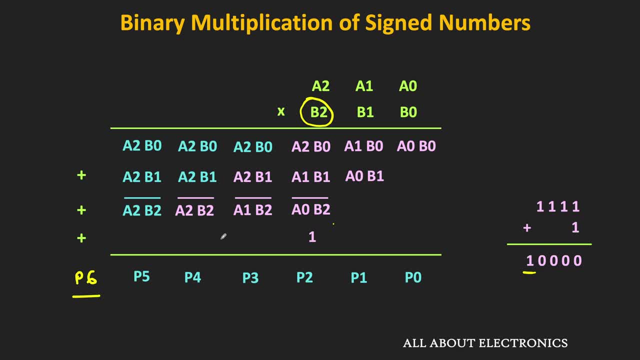 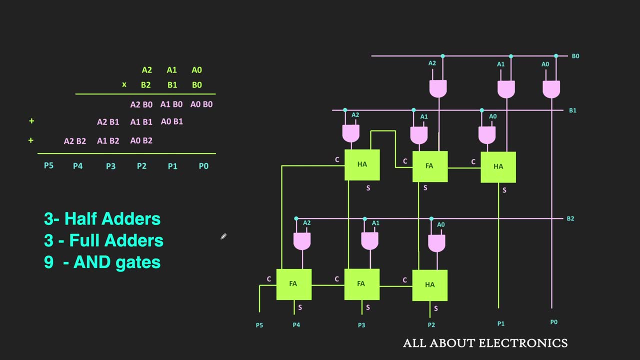 unsigned binary multiplier. here we require the additional hardware. So for the 3-bit unsigned binary number we require the additional hardware. And for the unsigned binary numbers we have seen that we require the 3 half adders, 3 full adders and the 9 and gates. 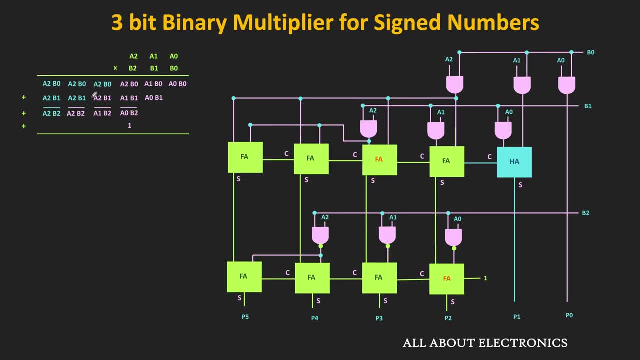 But in case of the signed binary multiplication, since we need to extend the signed bit of each partial product, so we also need additional full adders. So here this is the circuit of the signed binary multiplication of the 3 bit numbers. So as you can see over here, for this signed extension we require these additional full. 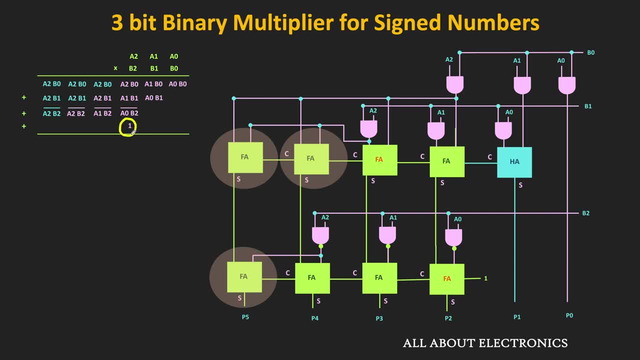 adders. Apart from that, for adding this one. Instead of the half adder over here we require the full adder. And apart from that, to complement these bits in the partial product: instead of the and gate, here the and gates are used. 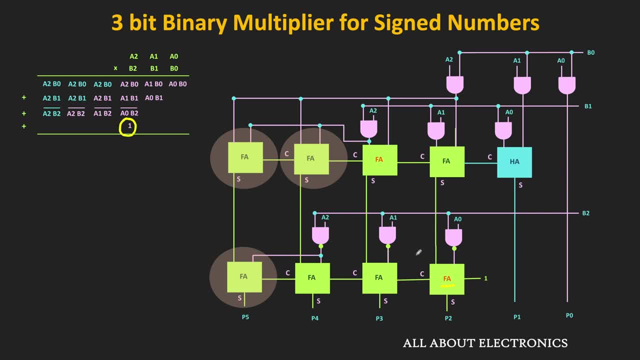 So, in short, for doing this signed binary multiplication we need the additional hardware in terms of the adders, And as the number of bits in the number increases, then we require the additional hardware. But with the little modification in the circuit we can avoid these additional adders which 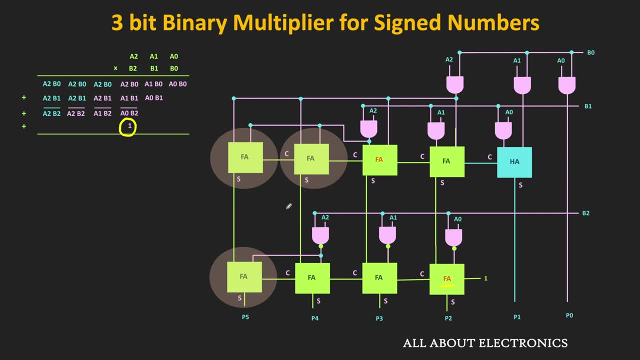 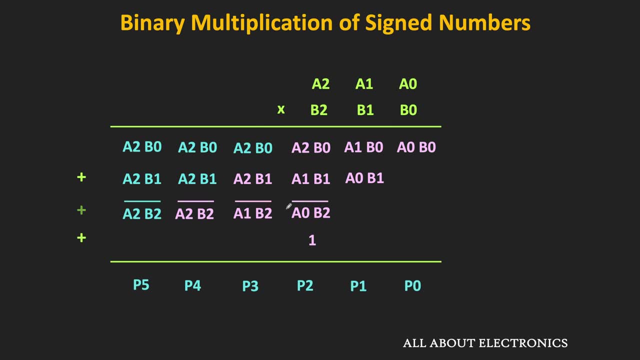 is required because of the signed extension. So let's see that. So here once again, the multiplication of the 3 bit signed number is shown Now. in this multiplication, at the 3 different locations the 1 is added and subtracted. 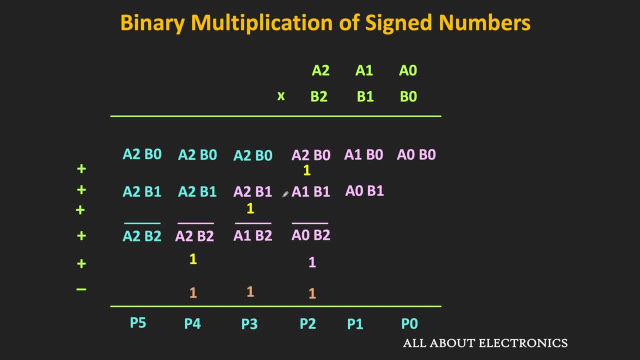 So if you see over here, then in the 3 different columns the 1 is added and the subtracted. So overall the multiplication will remain the same, But because of this operation now these additional signed extension bits will get vanished. 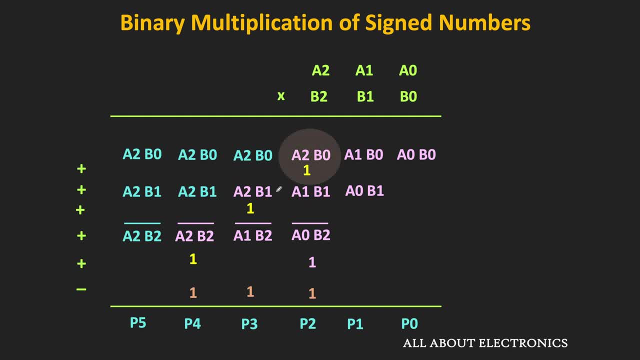 So let's see how. So first of all, let's see this 1, which is added with the a2b0.. So if the a2b0 is equal to 0, then after adding the 1,, the result will be equal to 1.. 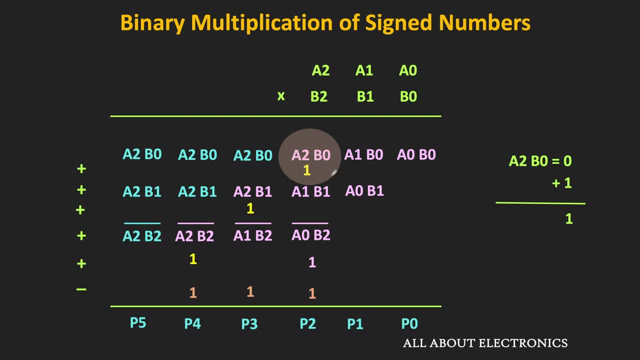 That means, at this position, we will have 1.. But since the a2b0 itself is equal to 0, so all the signed extension bits will be equal to 0. And since they are 0, so there is no point of writing them. 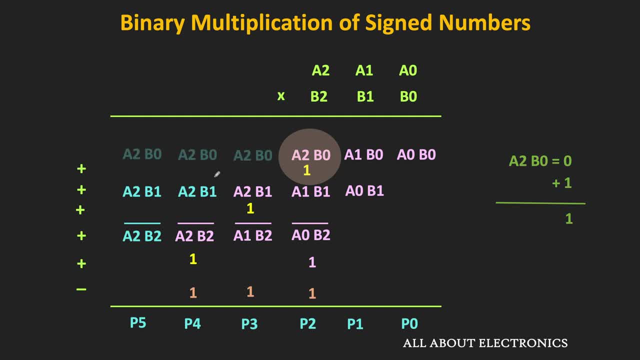 On the other end, It will be the same thing when this a2b0 is equal to 1.. So if the a2b0 is equal to 1, then after adding this 1, the sum will be equal to 0,. while. 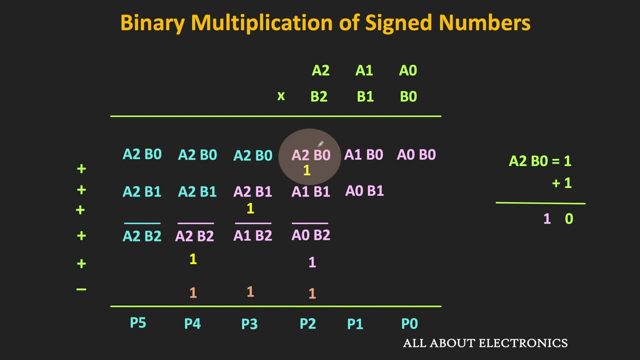 the carry will be equal to 1.. That means now at this location we will have 0. And this carry will be forwarded to the next stage. So once again in the next column, this a2b0 is equal to 1.. 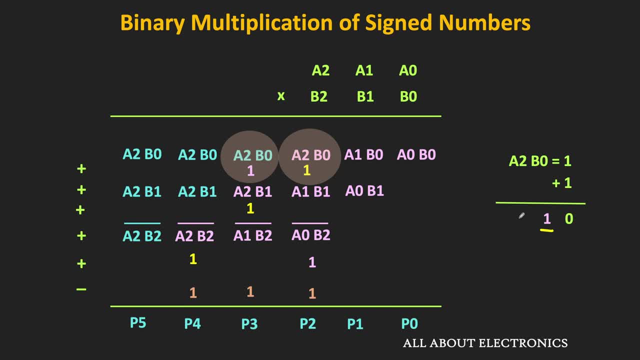 Therefore, this 1 plus 1 is equal to 0. And there will be a carry of 1. And once again it will be forwarded to the next column. So once again, in the next column, this 1 plus 1 is equal to 0 and 1 will be the carry. 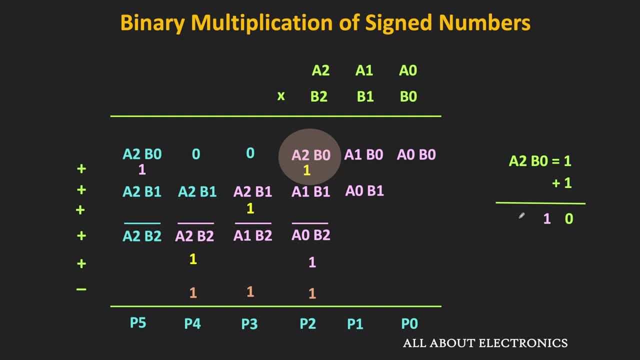 So once again it will get forwarded to the next column And once again in the next column this 1 plus 1 is equal to 0 and 1 will be the carry. But now, if you see, then this carry will be at the P6 position. 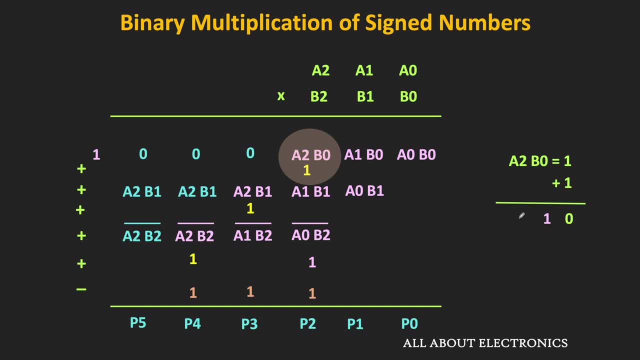 But here, since we are only concerned about the first 6 bits or in general for the first 2n bits of the multiplication, so we can ignore this P6 bit. So, as you can see, even if the A2B0 is equal to 1, then also after the addition of the 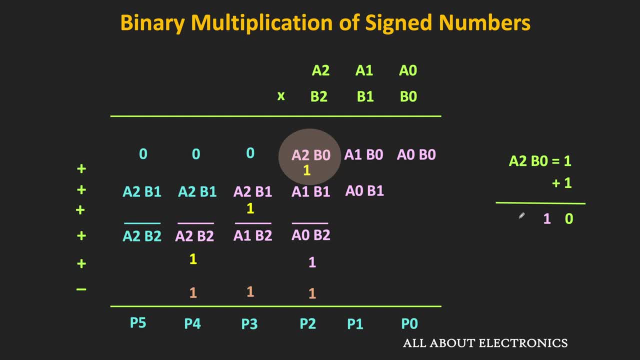 1,, all the sign extension bits will become 0. And since they are 0, so there is no point of writing them. So in general, we can say that when we add this 1 to this A2B0 bit, then irrespective. 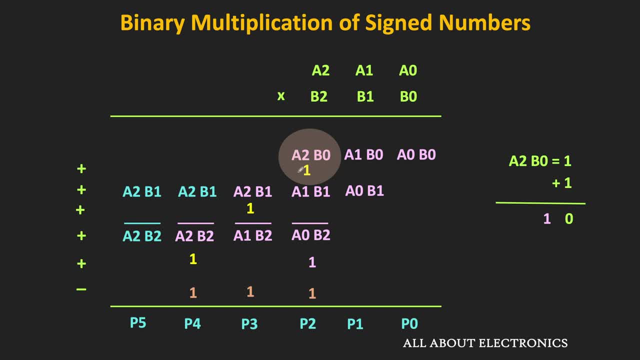 of the value of this A2B0.. All the sign extension bits will get vanished. Moreover, after the addition, this A2B0 bit, at this position, will get inverted Because, as we have seen, if this A2B0 is 0, then after adding this 1, the result will 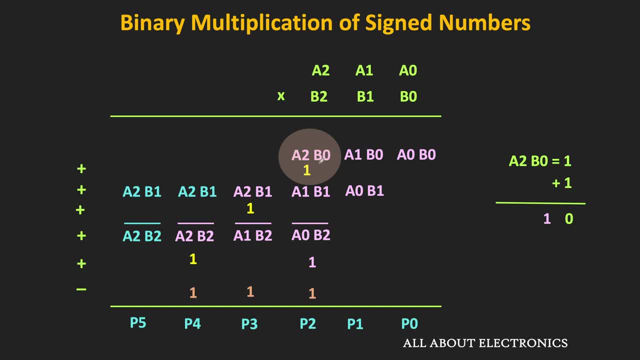 be equal to 1, which is the complement of the A2B0.. And similarly, if this A2B0 is equal to 1, then after adding this 1, the result will be equal to 0, which is, once again, the complement of this A2B0. 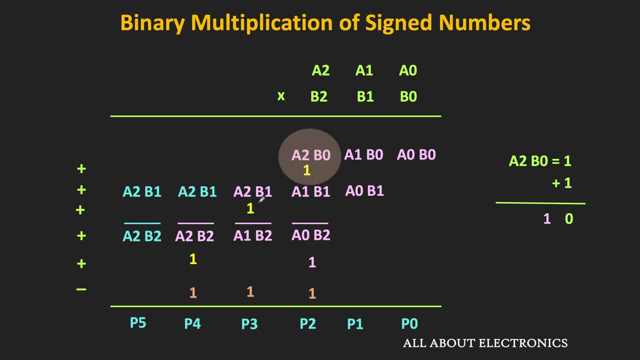 That means, in short, this A2B0 bit at this position will get inverted. And similarly, with the same logic, when we add 1 to this A2B1 bit, then all the sign extension bits will get vanished And this A2B1 bit will get inverted. 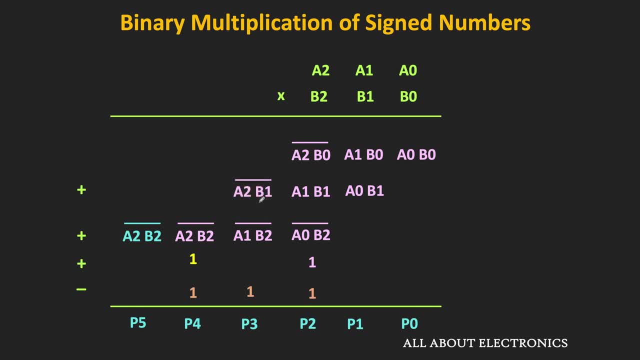 Similarly, when we add 1 to this A2B2 bar, then the sign extension bit will get vanished And this A2B2 bar will get inverted. Now here this –111 is equivalent of 1.. Now this 2.. 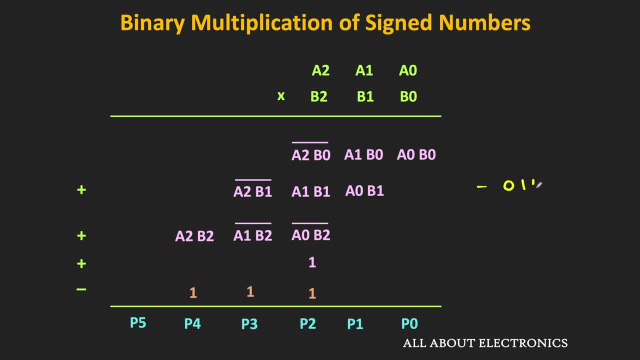 This 2.. This 2.. So if we take the 2's complement of this number, then this minus sign will get converted to the plus sign And, as you know, the 2's complement of this number is equal to 1001.. 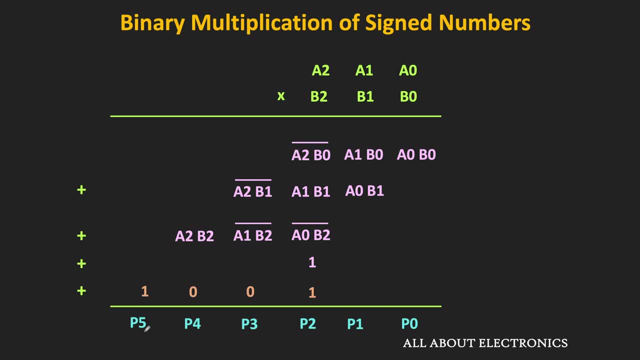 So of course, over here, while performing the 2's complement, we are considering the bits only up to the P5 location, Or, in general, we are considering the bits up to the 2nd location. So now, when we add 1 to this 1001,, then the result is equal to 1010. 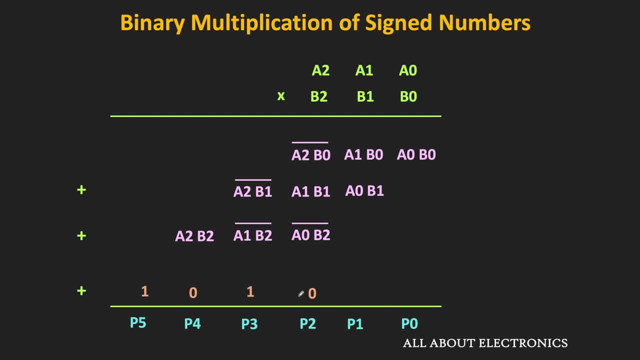 So, basically, in terms of the hardware, if you see, then we need to add the 1 at the P5 and the P3 locations. So now, if you think, in terms of the implementation, then we need to invert these 4 bits and we 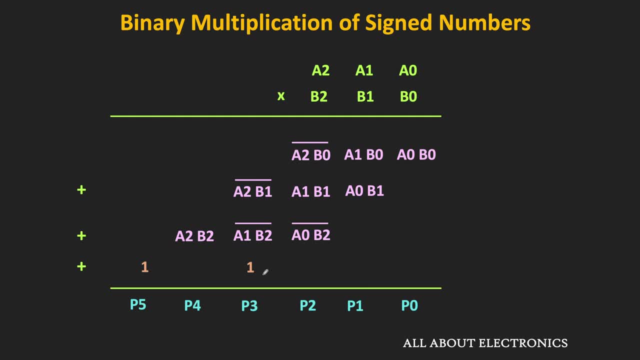 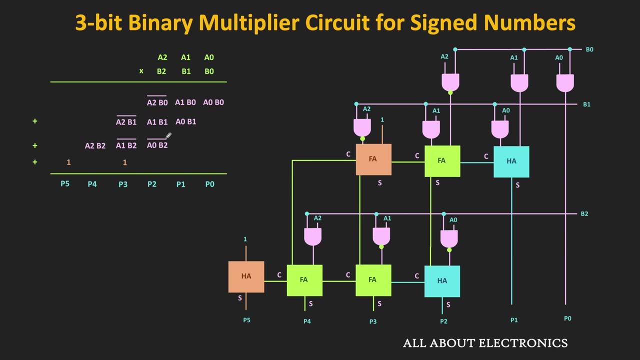 need to add 1 at these 2 locations. So this is the modified circuit of the 3-bit multiplier for the signed numbers. So, as you can see, To invert these 4 bits, instead of the AND gate the NAND gates are used. 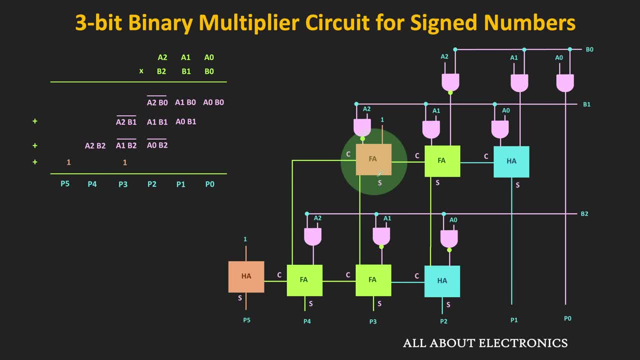 And here to add the 1. at this P3 location, instead of the half adder the full adder is used. So if you recall the 3-bit multiplier for the unsigned numbers, then at this location we have used half adder. 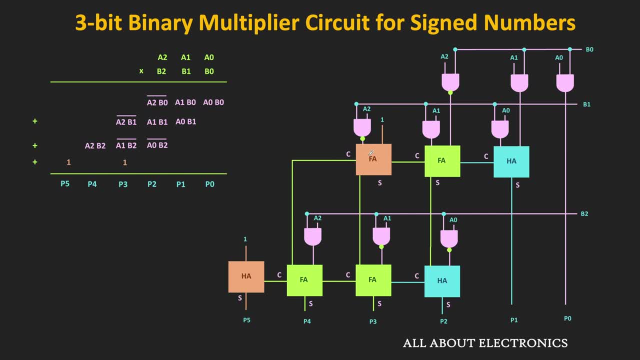 But here to add this additional 1, we have used full adder And similarly, using this additional half adder, this 1 at the P5 location can be added. So in this way, by using the minimum additional hardware, we can use the same multiplier circuit. 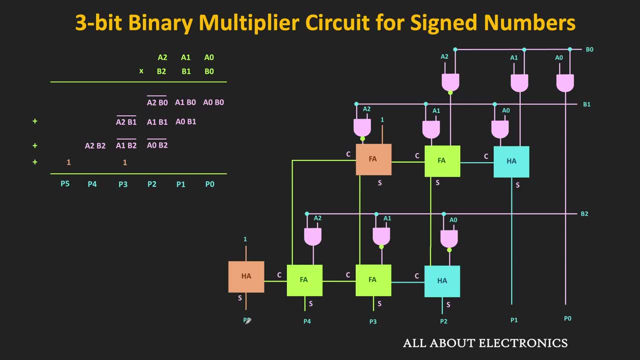 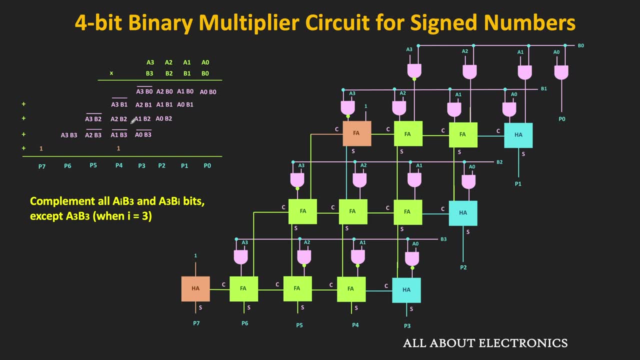 for the signed numbers. So similarly, this is the circuit of the 4-bit multiplier for the signed binary numbers. So basically, over here we need to complement all the A3Bi and the Eib3 bits, except when i is equal to 3.. 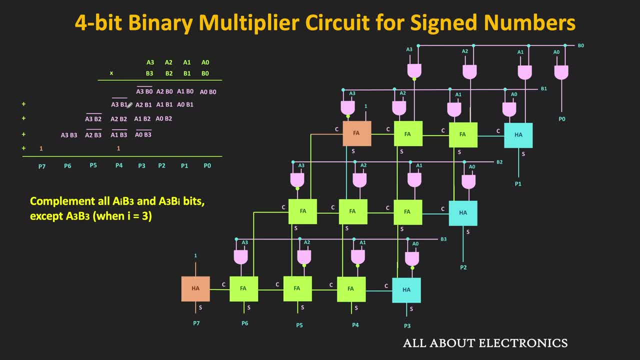 That means here these A3B0, A3B1 and A3B2 are complemented. Similarly these A2B3, A1B3 and A0B3 are complemented. So this is the 3-bit multiplier. So the A3B1 and A3B2, both are complemented. So in this way we can use the same B3 for the signed numbers. Similarly, this A3B0, A3B1 and A3B2 are complemented. 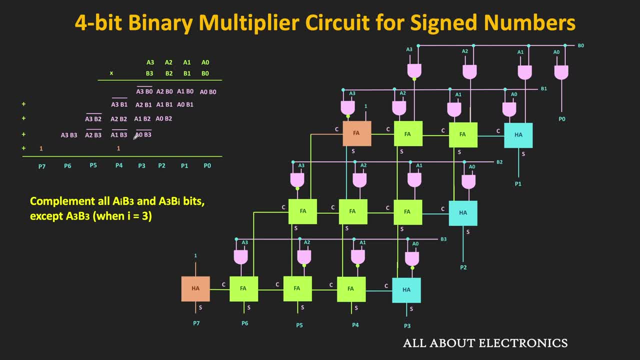 Similarly, this A2, B3, A1, B3 and A0, B3 are complemented. So, for example, if we have a 5-bit binary multiplier, then each binary number will have 5 bits. So in that case we need to complement all the AIB4 and the A4BI bits, except when i is. 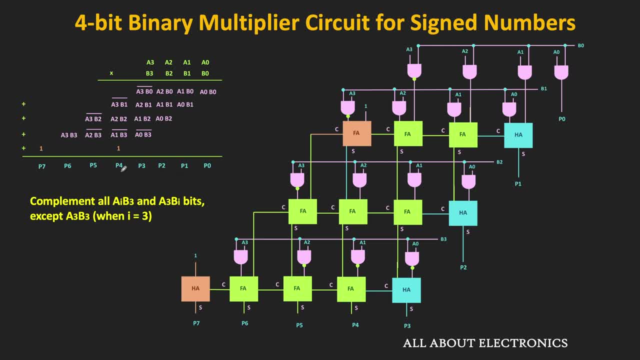 equal to 4.. So here, in case of this 4-bit binary multiplier, all these 6 bits are inverted And after that we need to add the 1 at this n plus 1 and the 2n locations. So for this 4-bit multiplier, starting from the LSB, we need to add the 1 at the 5th and